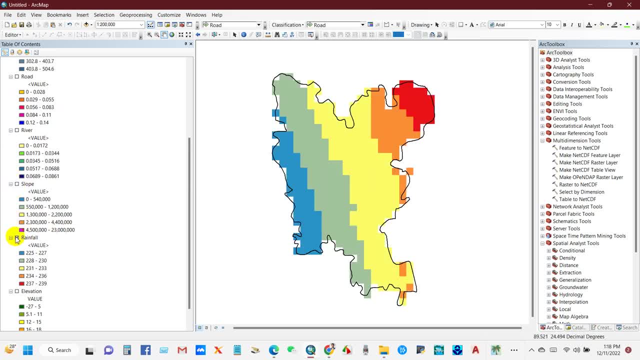 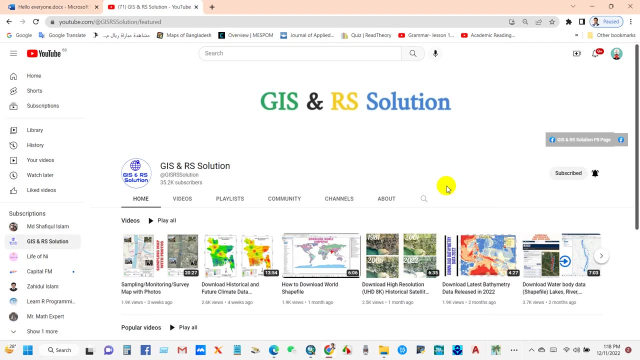 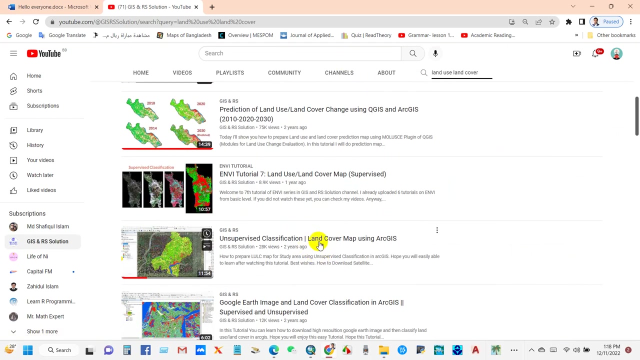 then you can see here rainfall and you can see over here elevation. so i have prepared these variables using js- i mean arcjs- and now i will show you how you can find these variables and how you can prepare this variable. so for that you will find all the variables how you can prepare. i am in my channel, so just go to. 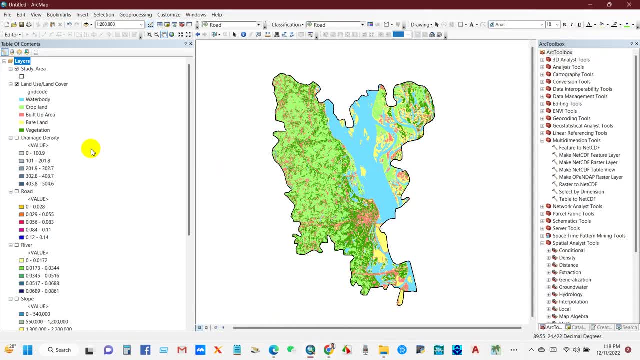 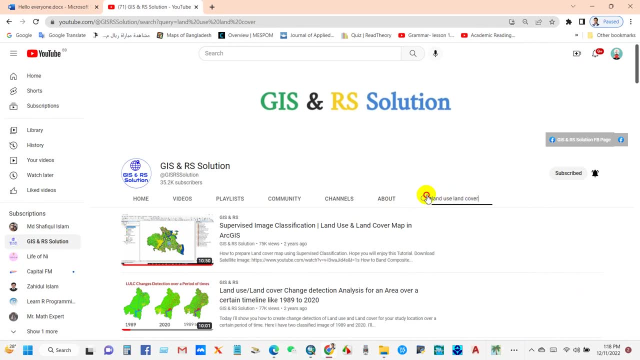 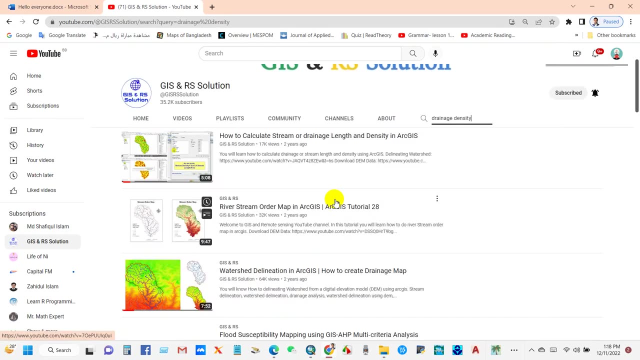 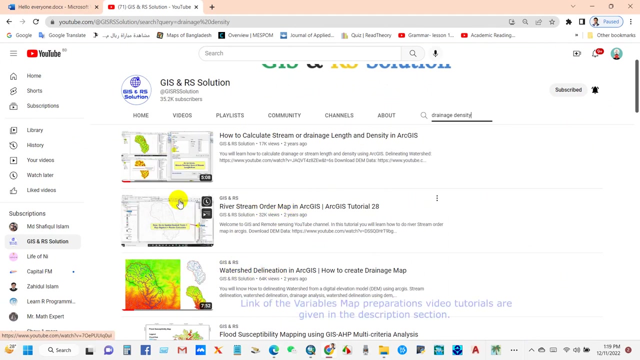 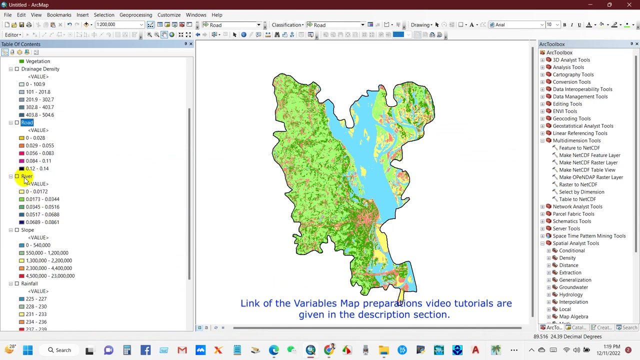 search box. after going to my channel and search the variable name, you will find everything in my channel, for example drainage density. just search drainage density, you will find the drainage density, watershed delineation, river stream order map. and also if you search distance from road, distance from river slope, rainfall elevation, you will find. 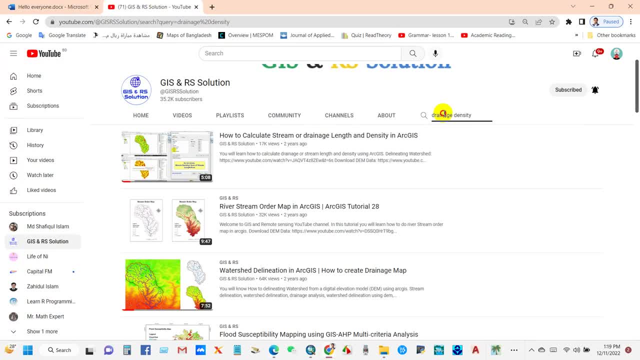 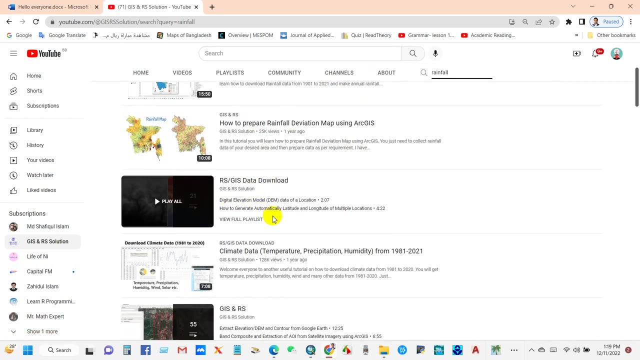 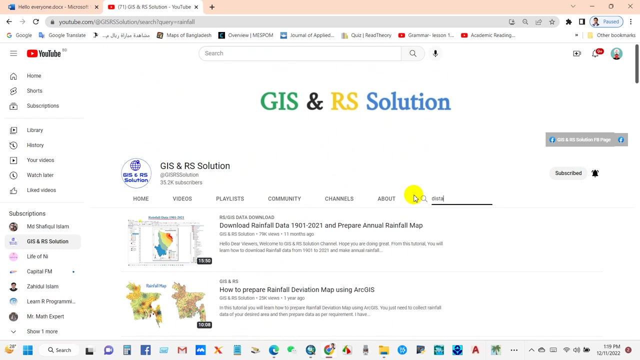 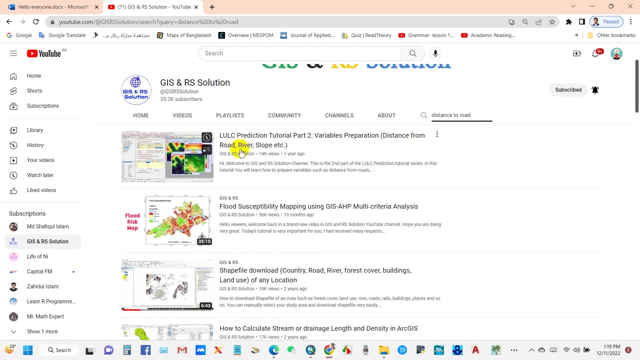 every, every, everything. in my channel, for instance, i'm writing rainfall and after that you will find several video about how you can prepare a rainfall map. or if i search writing distance to road, then you will find a tutorial. we have a preparation. distance from road- river slope. 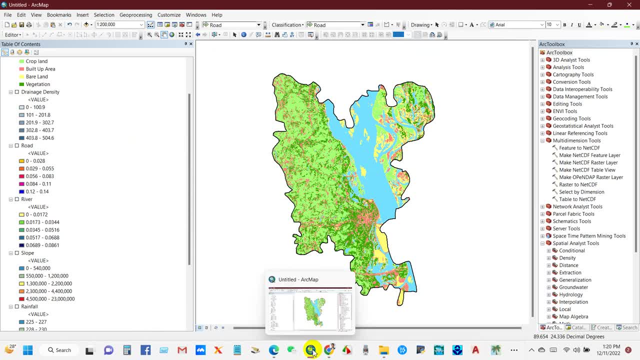 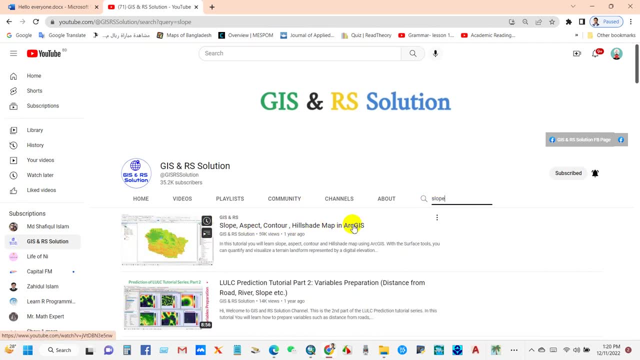 similarly, you will find every variables preparation technique in this channel, like slope. so i think i think this video can be very helpful and useful to you guys. so i hope you have enjoyed the video. please subscribe to my channel and leave a comment. see you in next video. see you, bye, bye, bye. 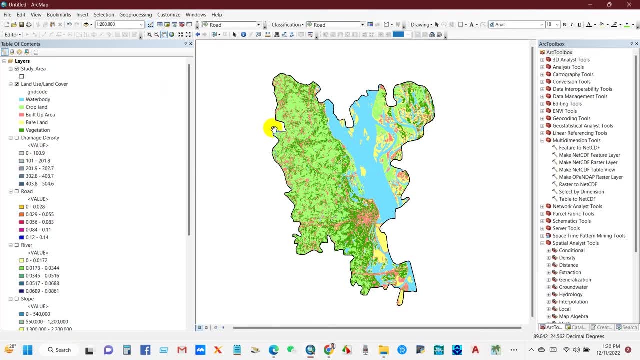 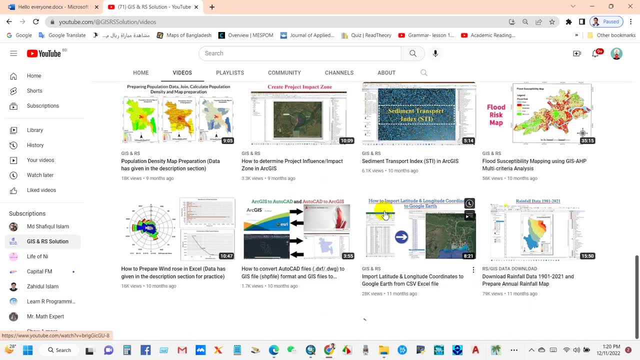 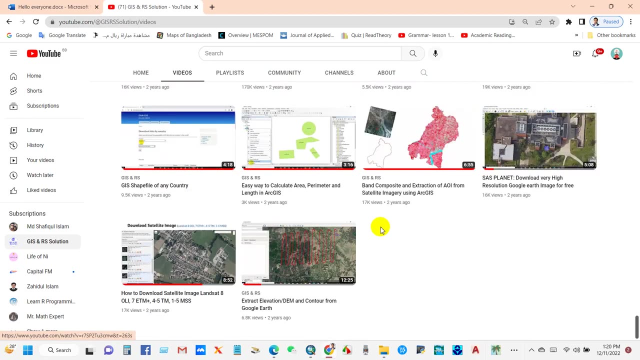 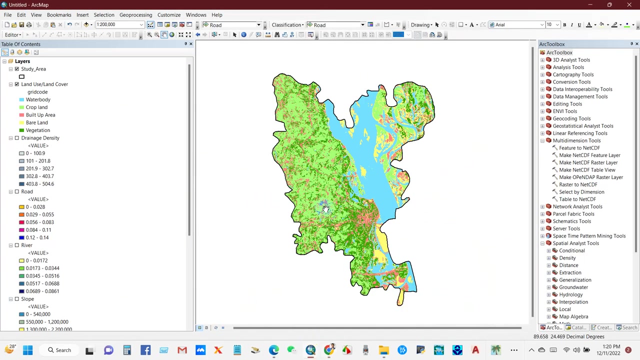 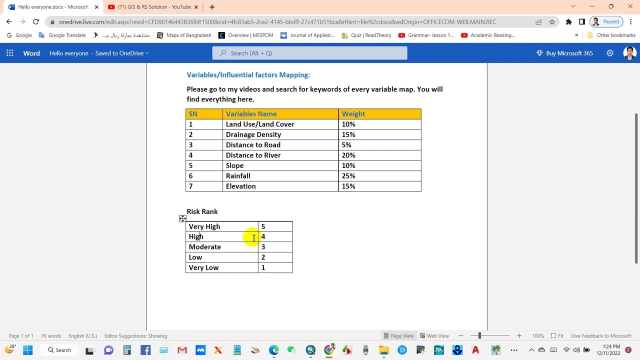 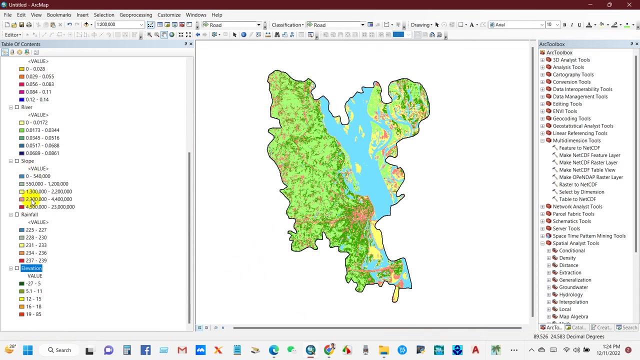 will find this helpful to reduce time consume, consume consuming. I have already prepared this variables, so I hope you will find this variables here how you can prepare. after preparing all the variables, you can see here the risk rank. I have ranked the risk 5 to 1. 5 means very high and 1 very low. and now I will 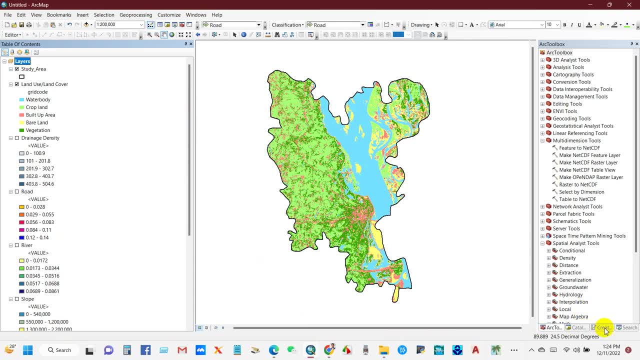 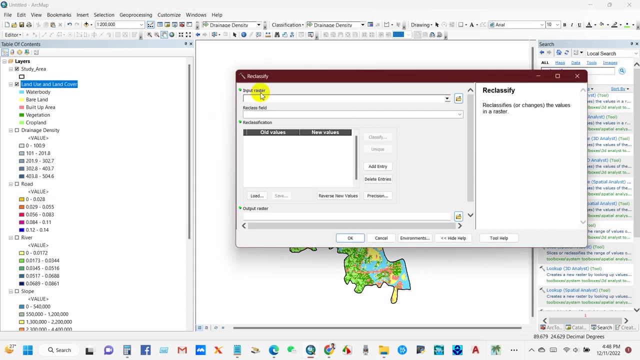 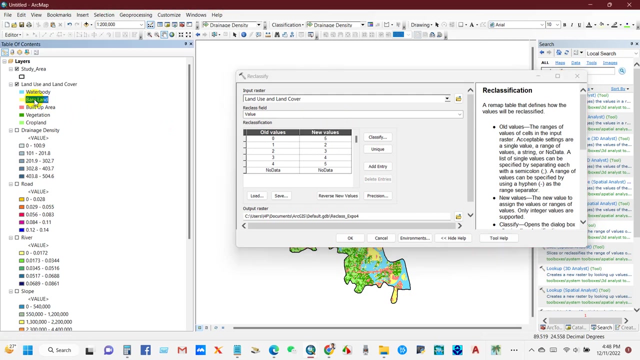 reclassify all the variables. so for that go to search box and write reclassify and then search. you will find here reclassify a special analyzed and then input raster will be the variable, like land use and land cover. here you have to set the new value, I mean the risk factor, I mean the water body, the high influence, one flat I mean. 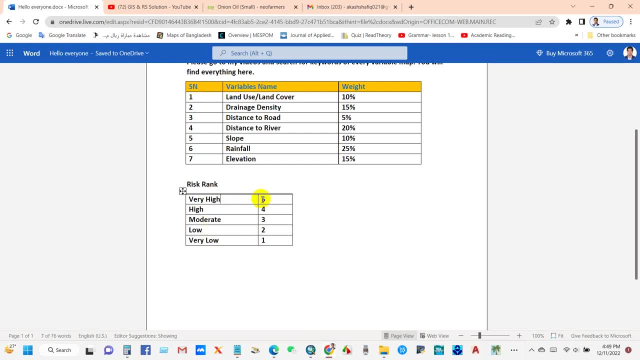 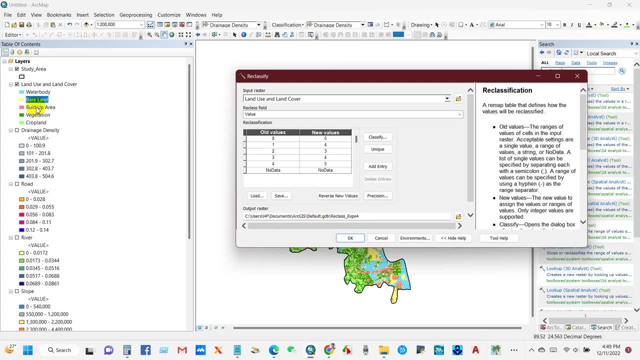 very high. I mean the water body, the high influence, one flat I mean very high risk for water body and then balance. it is a. I have given for and then built up, have given for and then built up, given three: the moderate and for vegetation I have given a very low and 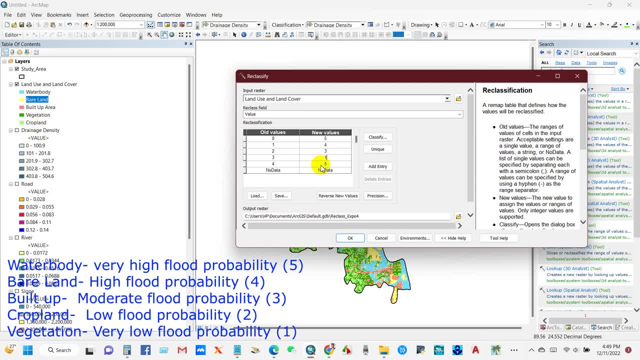 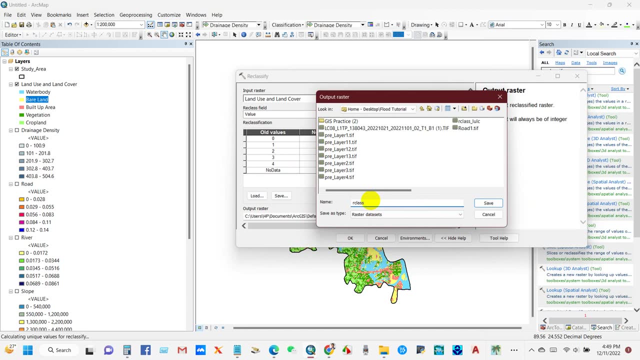 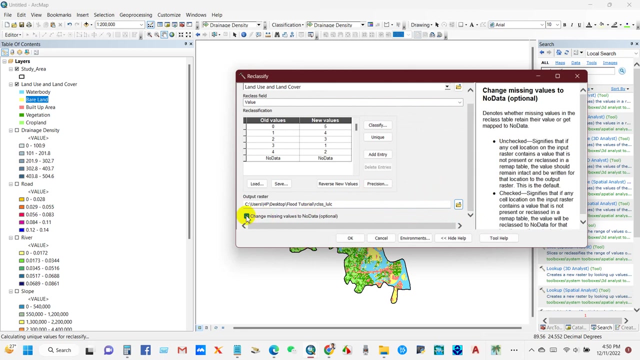 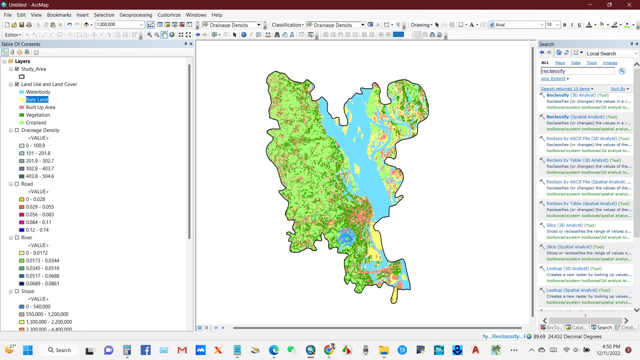 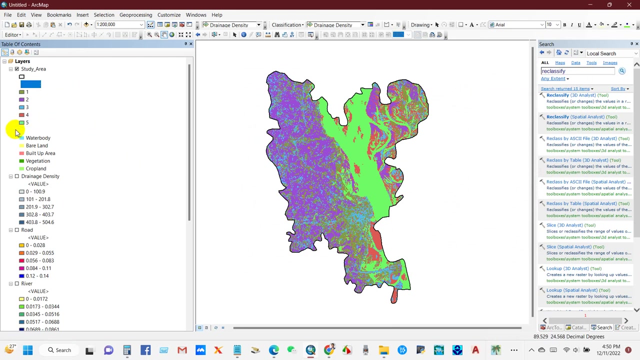 given three, the moderate and for vegetation I have given a very low and plant to I mean low probability for flat. it influences on flat happening. and then save the output raster, change missing values to no data, check this on and then okay, and I have classified LLC according to risk factor for flat, and then again, 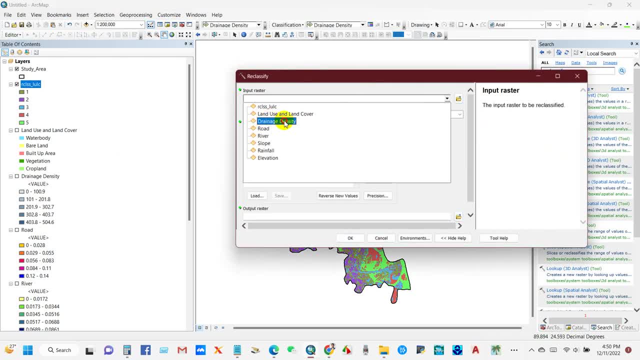 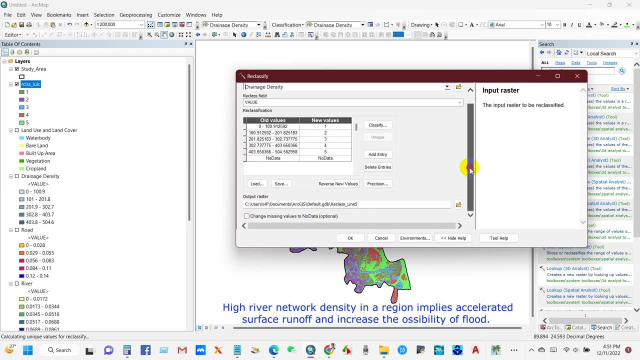 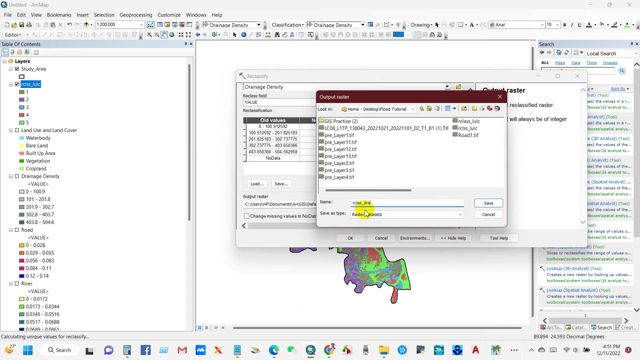 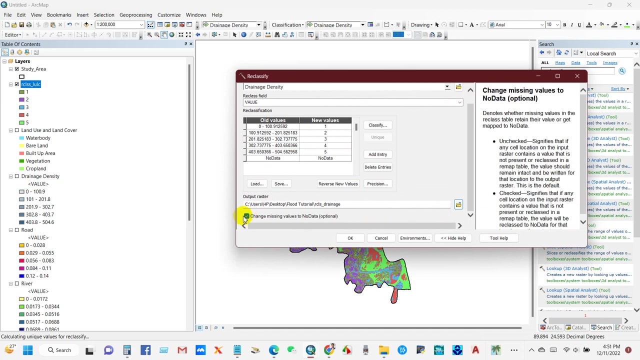 reclassify and then drainage density. drainage density I mean the higher drainage density means higher flood risk. so it it has been already arranged. one to five: I mean very low to high risk. that means lower density means low flood probability and higher density means high, higher flood probability. so output raster, save our to raster and then check change missing. 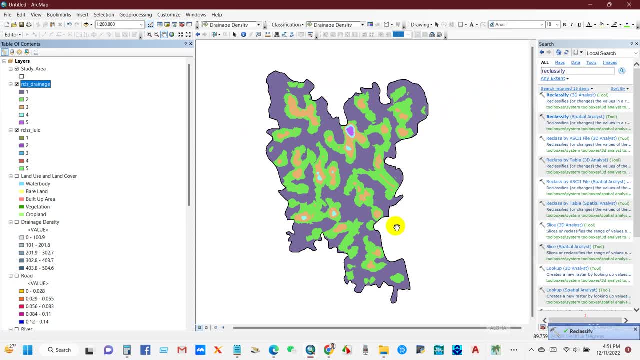 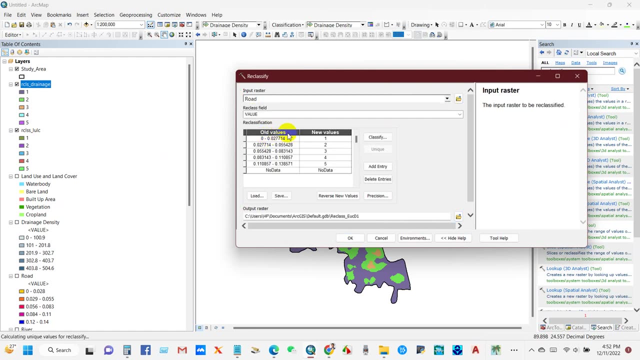 values. and then okay, and it has also done for drainage density- one to five, and then again reclassify and this time it will be a road distance from road, so very close to the road distance. really that means very high flat probability. so reverse new values five to one. 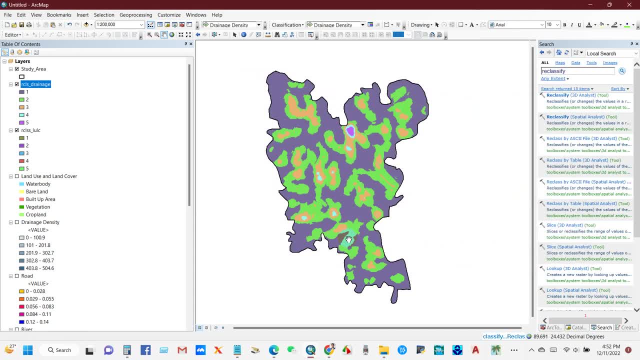 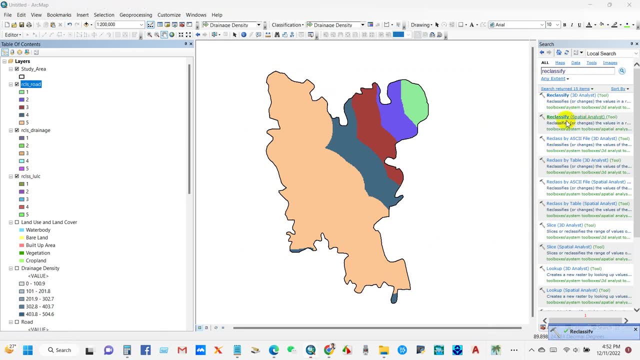 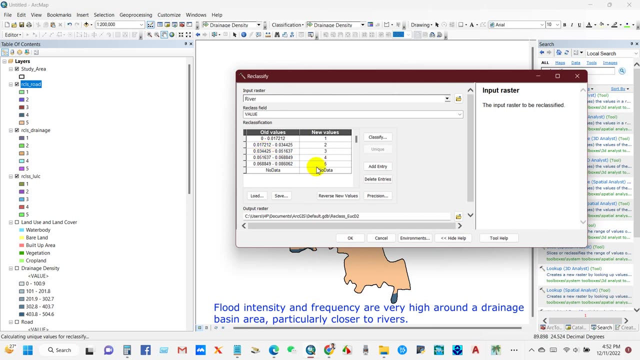 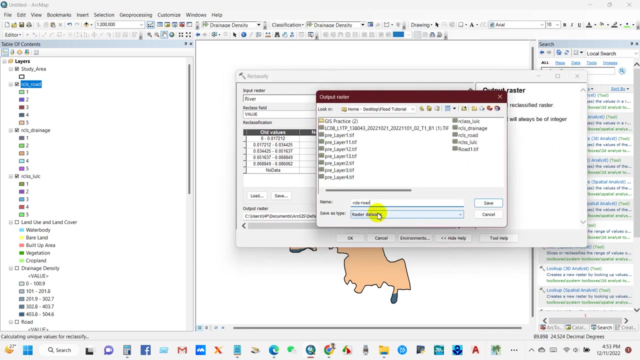 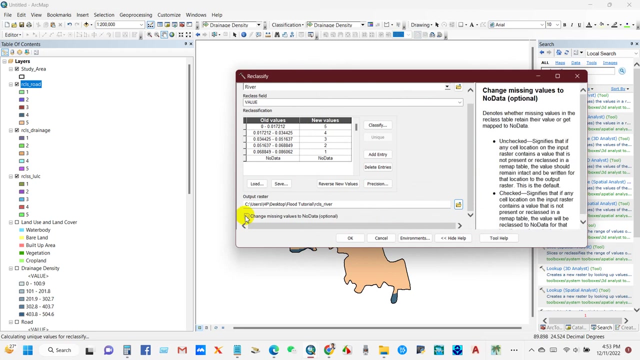 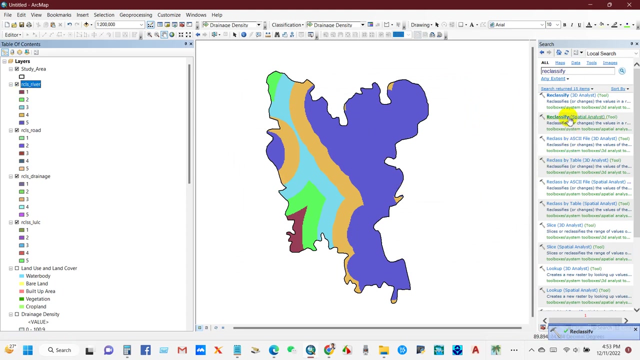 and then click OK. and then again for river distance from river. the shorter distance means high flat probability, so this time it will be also five to one. I mean the distance increases, the flood probability will be decreases. I mean the close to the river means higher file flat probability. and then: 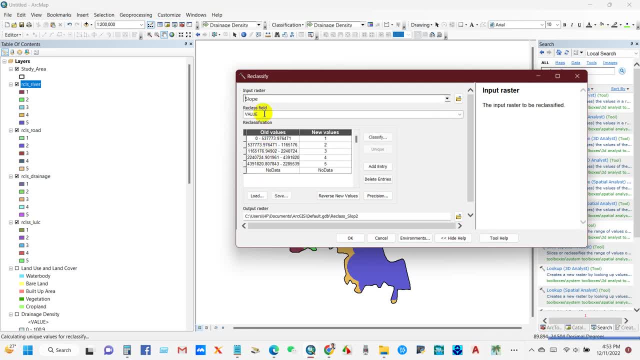 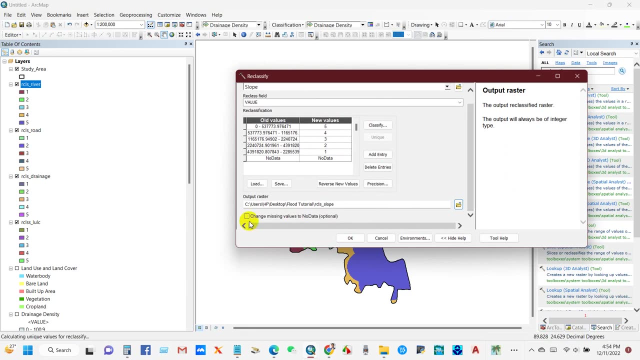 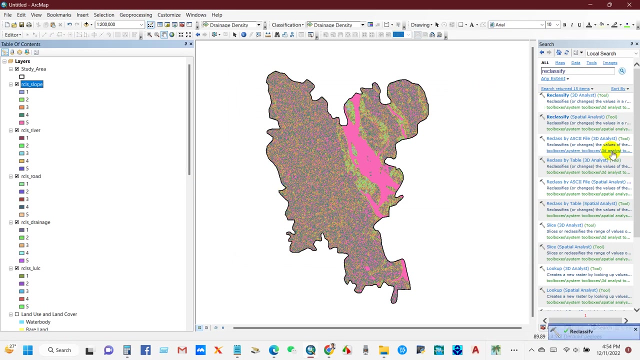 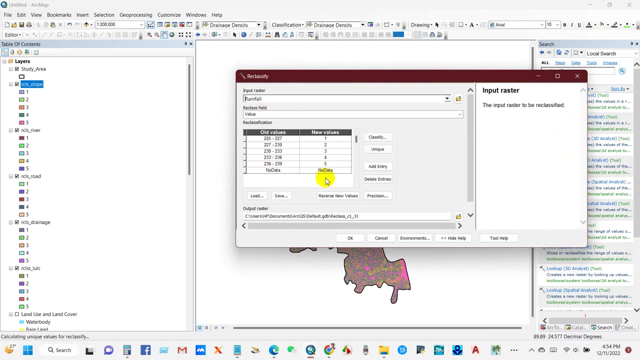 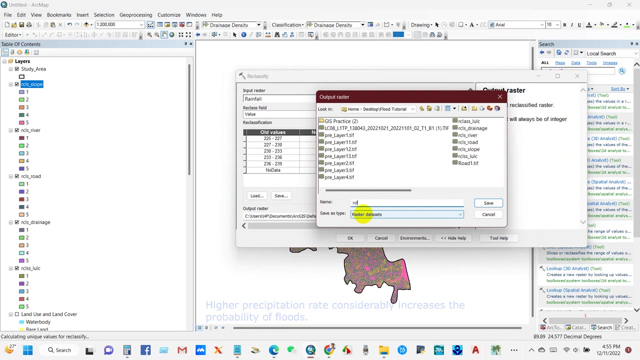 for all slope it will be a reverse also. and then for slope it will be a reverse also: higher degree slope means low flood probability. and then for rainfall. so higher rainfall means high fall flat probability. so lower rainfall means lower low flood probability. so it will be one, two, three, four, five, six, seven, eight, nine. 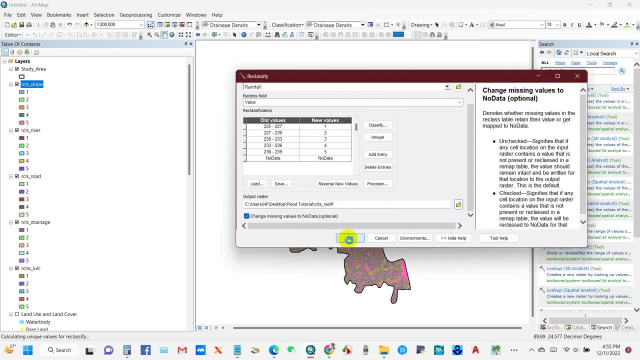 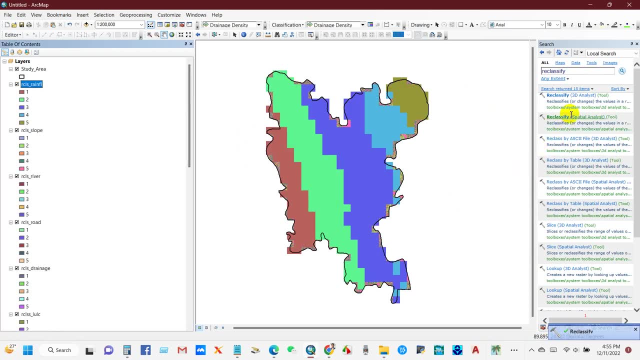 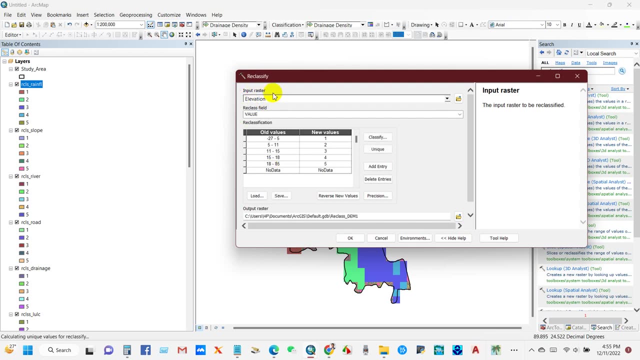 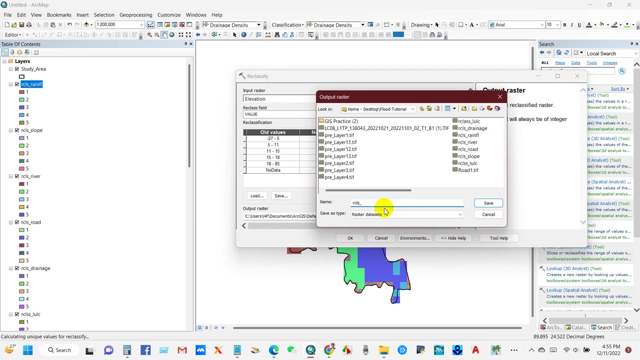 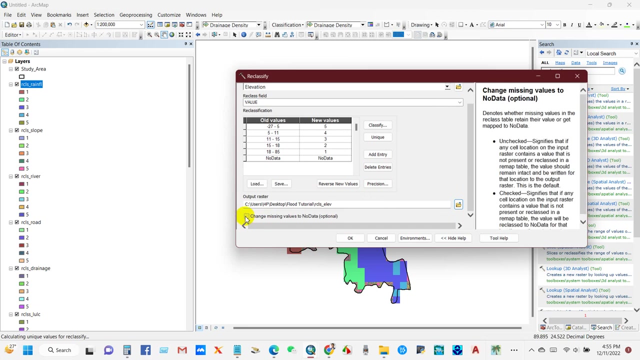 two, five- very low to very high risk, and then again reclassify and input raster elevation, and here low elevation means higher flood probability and high elevation means lower flood probability. so it will be five to one, very high to very low, and check this out and then okay. so 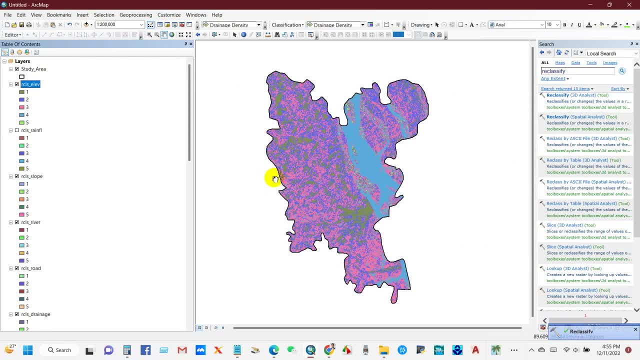 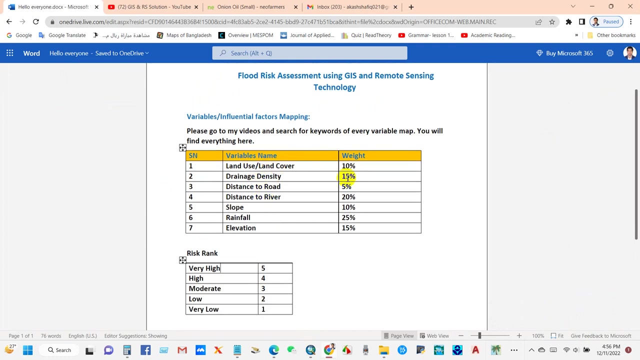 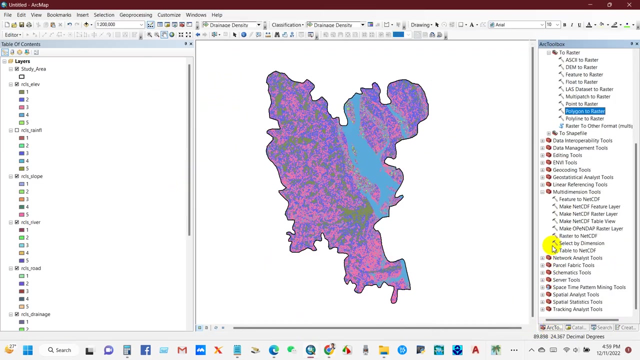 I have classified all the raster, all the variables, and I have ranked one to five: very low to very high or very high to very low. elevation, rainfall slope, reward, drainage density LLC. I have taken total seven variables or factors to identify flood risk and the important thing is weight and how you can weight. you can use ASP. 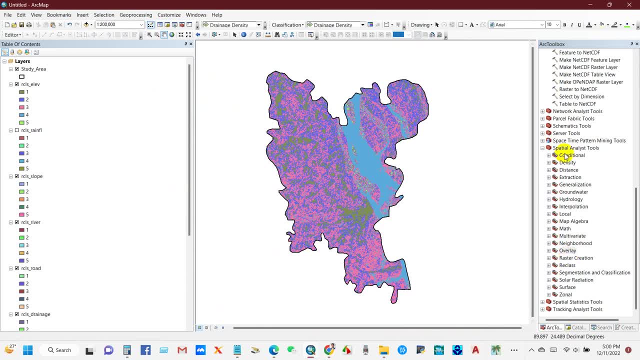 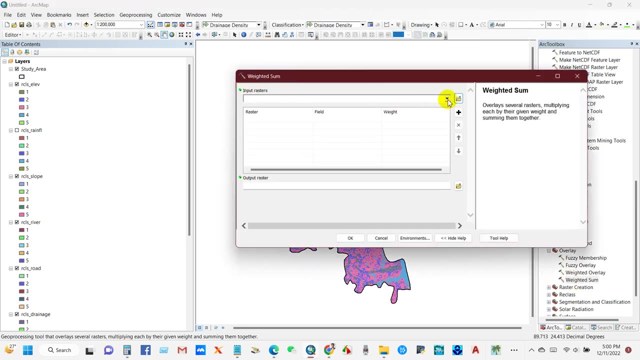 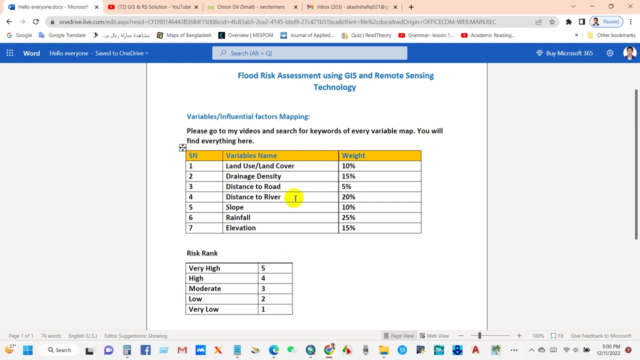 technique or use. I mean personal judgment or expert opinion. to weight for every factors here I have used weighted sum. you will find this from the special analysis toolbox. so for land use and land cover I have a. I have given 10% out of 100. for rainfall I have given 25% out of 100. and distance, 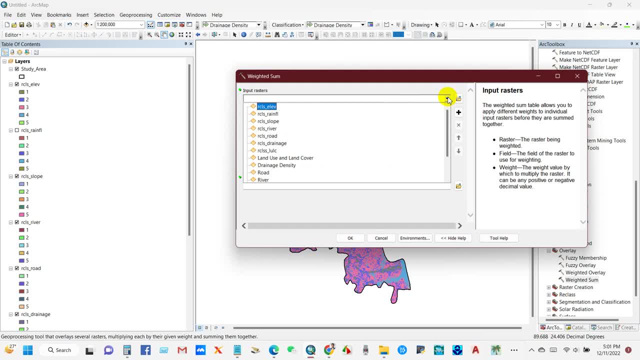 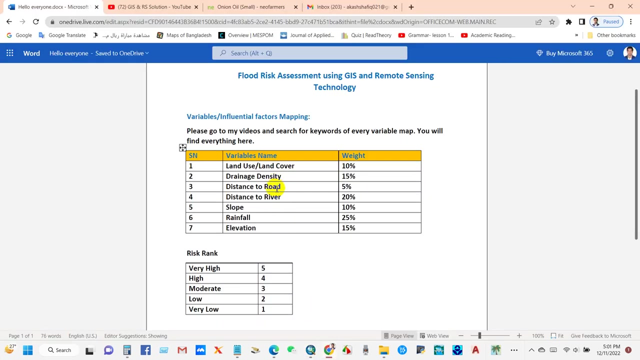 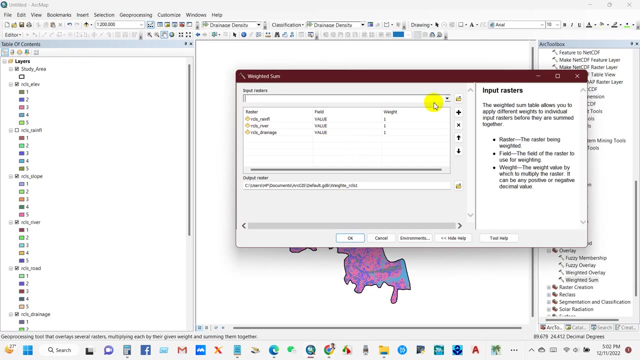 to river: 20%. so out of 100 you have to give in the percentage for every variables: the rainfall, River and elevation slope levels, e. so have added all the variables here, the weighted sum and now elevation slope level, see. so I have forget all the variables here in the weighted sum. and now 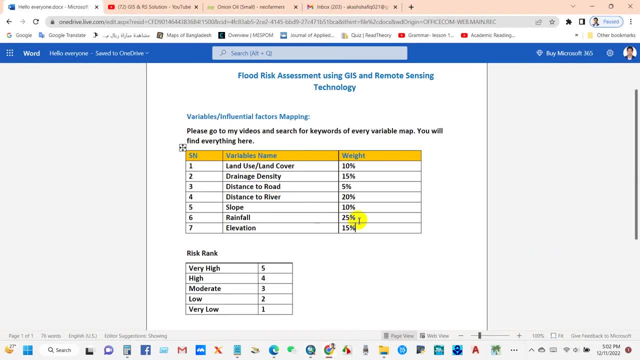 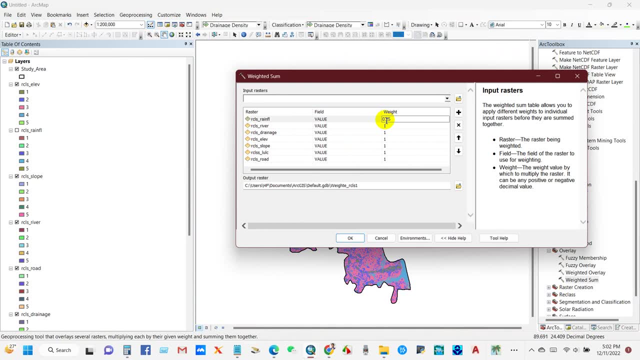 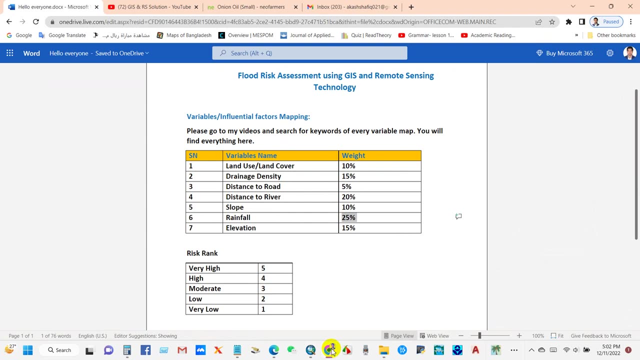 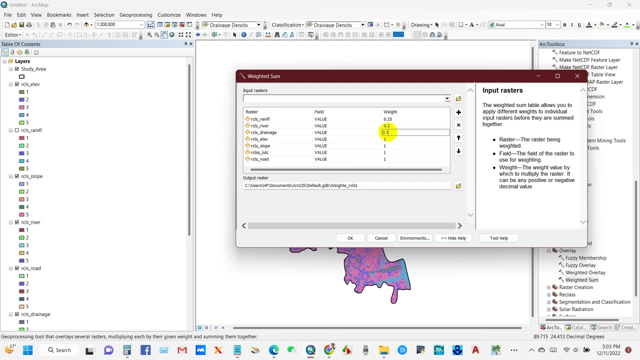 a will put the wet for rainfall, it will be 25 percent. so what will be? point zero to five? point twenty five percent and river it will twenty percent. point zero two and rain is density, it will also point zero on five and elevation, point zero on five.